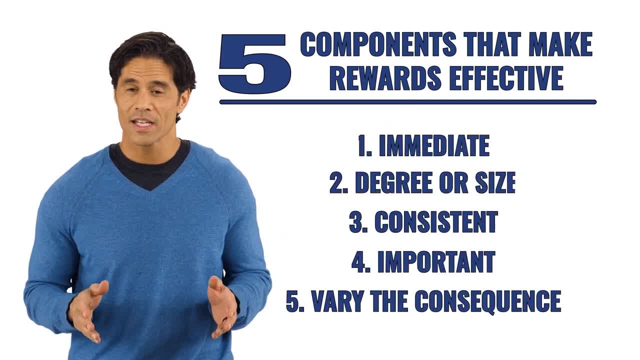 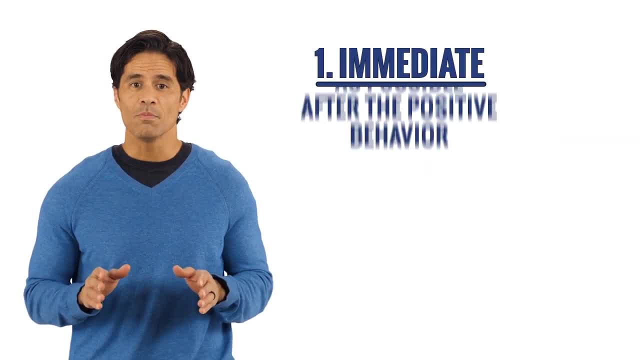 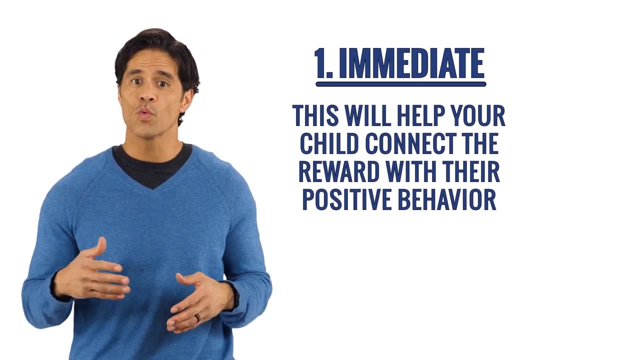 if a reward isn't working, it's because it's missing one of these components, or one of the components needs to be adjusted. immediate means the reward should be given as soon as possible after the positive behavior. this will help your child connect the reward with their positive 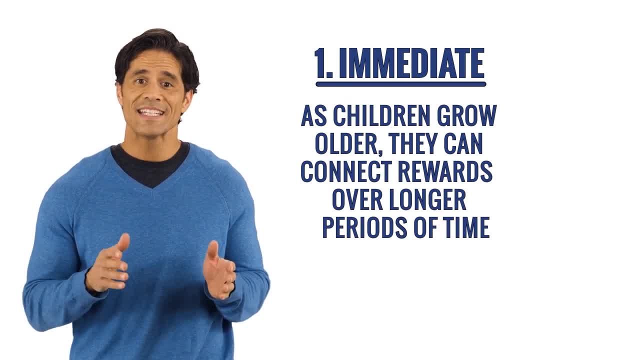 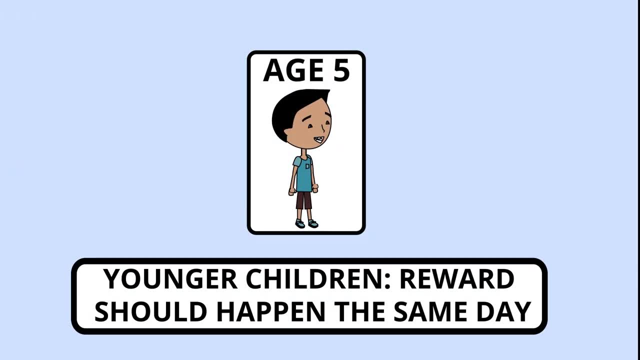 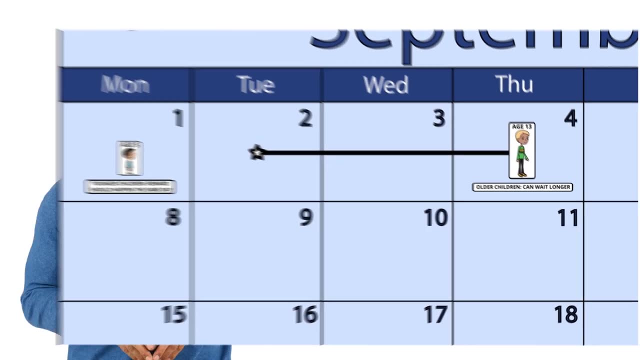 behavior. as children grow older, they can actually connect rewards over longer periods of time. here's a tip: little children benefit from rewards that happen the same day. older children can wait longer. you'll know the difference for what works best for your child degree. your size means how big. 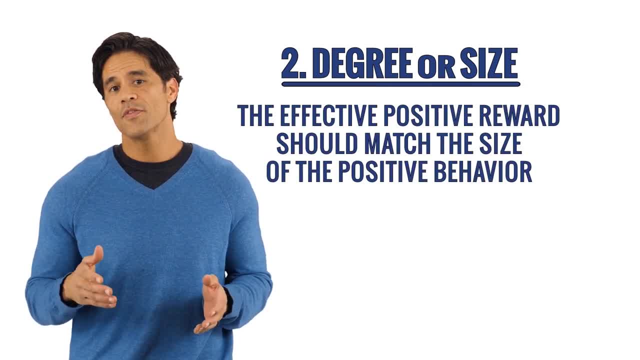 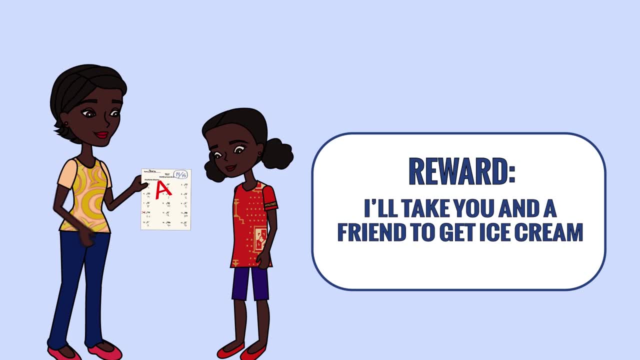 or small. the reward is based on what your child does. the effective reward should match the size of the positive behavior. here's a tip: it's better to give smaller, immediate rewards over time versus one huge one. it's better to give you a little number, smaller reward than a ark or size equivalent. 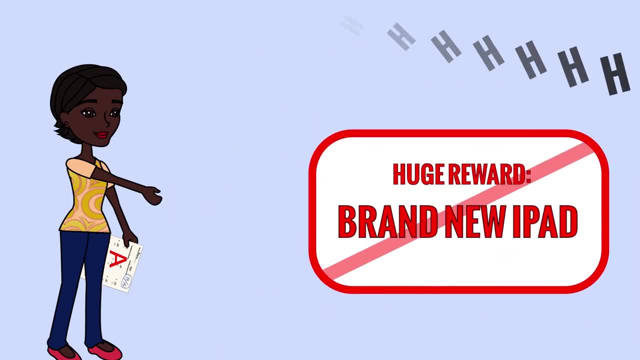 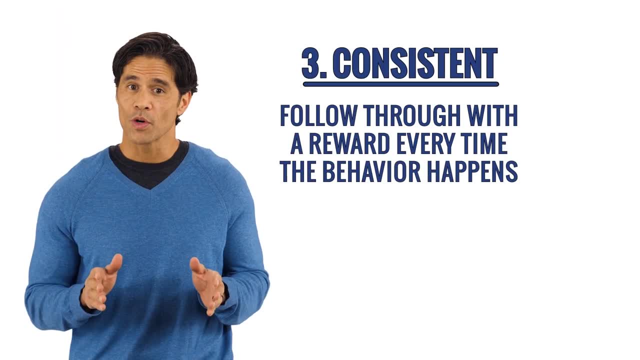 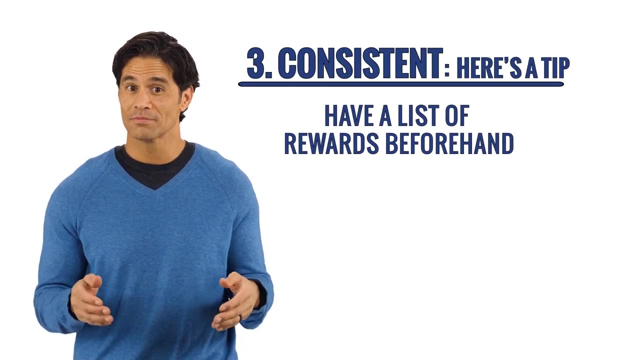 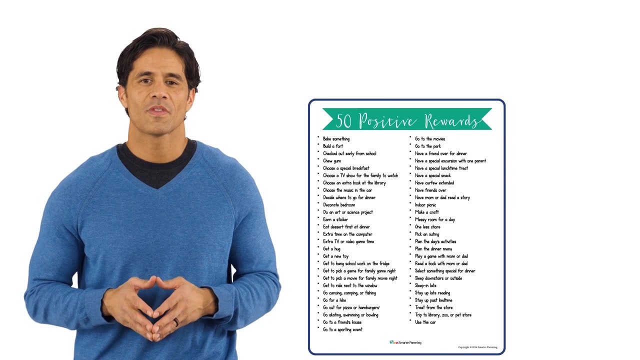 It is okay to keep rewards simple. Consistent means you follow through with a reward every time the behavior happens. Here's a tip: To be consistent, have a list of rewards beforehand. We have a list to help you on our website. Important means the effective rewards have to be meaningful to your child. 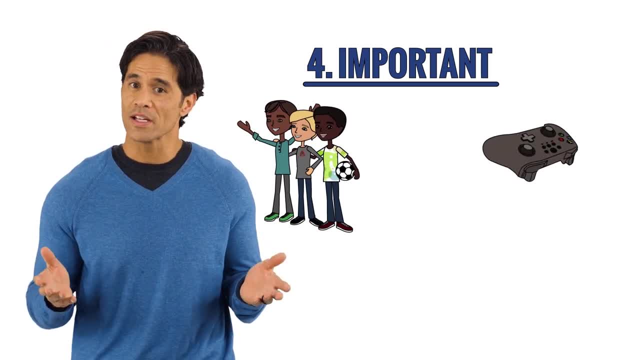 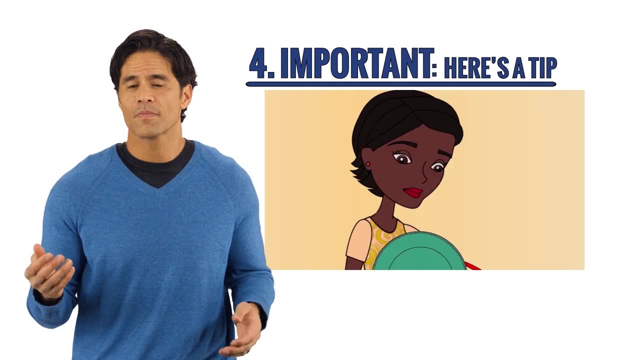 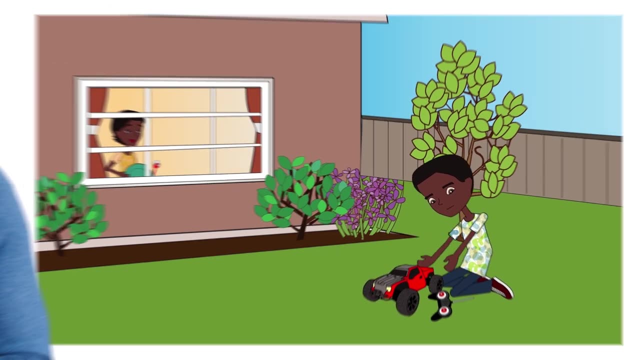 For example, allowing your child more time with friends. additional video game time or activities they enjoy can all be used as rewards. So here's a tip: You'll find what's meaningful to your child if you observe them, Watch what they do in their free time. 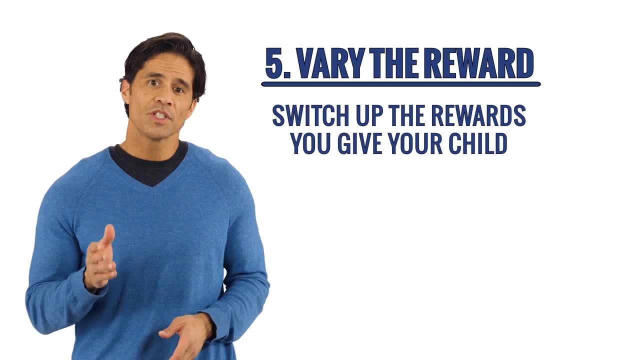 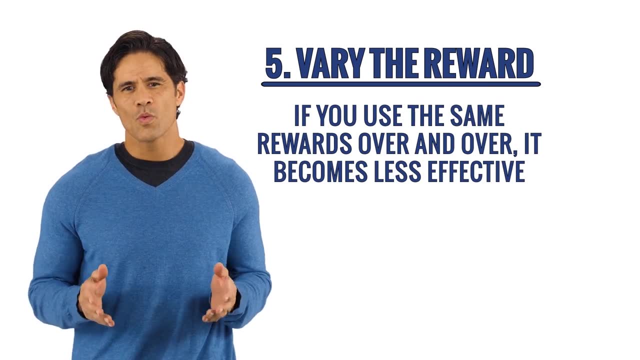 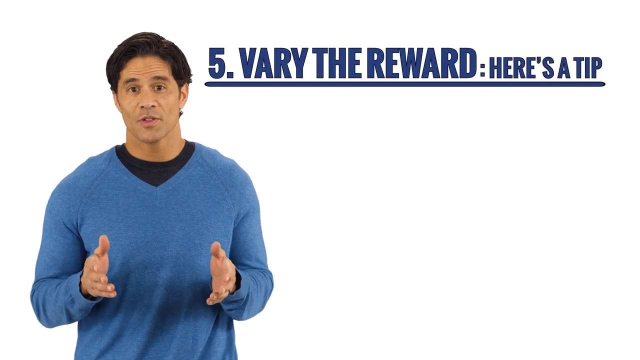 You will need to switch up the rewards you give your child. You should use a variety of rewards for positive behaviors. If you use the same rewards over and, over and over again for everything, rewards become less effective. Here's another tip: Understand that your child is going to change. 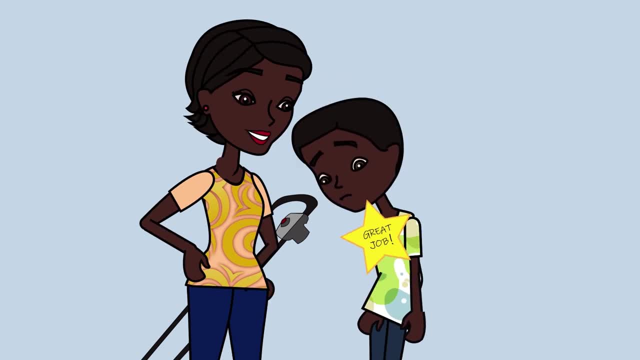 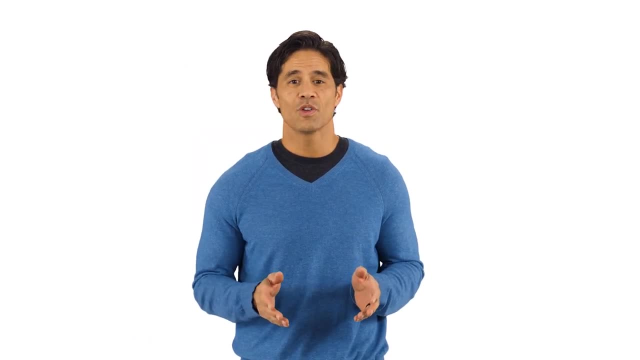 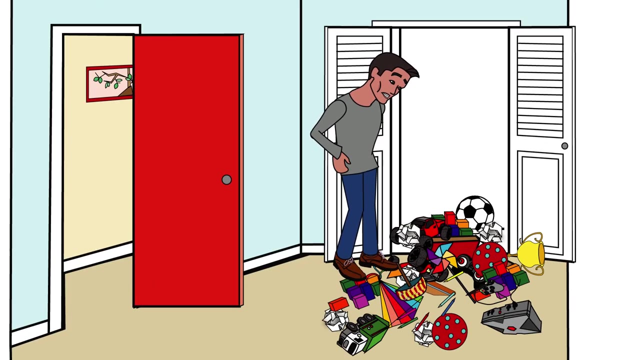 and you need to adjust rewards when it stops being effective. Giving your child a sticker isn't going to work forever. Let me tell you about a personal situation with my 10-year-old son, Michael. Michael and I had some problems because he used to lie to me about doing his chores. 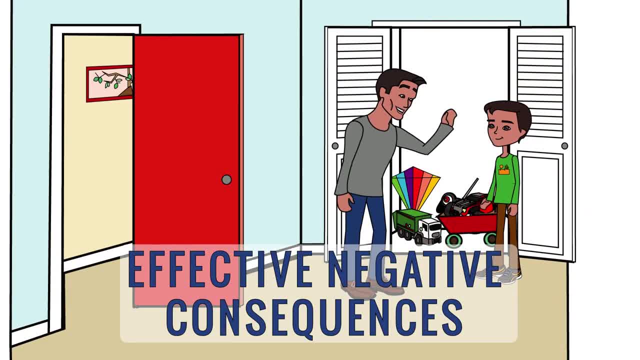 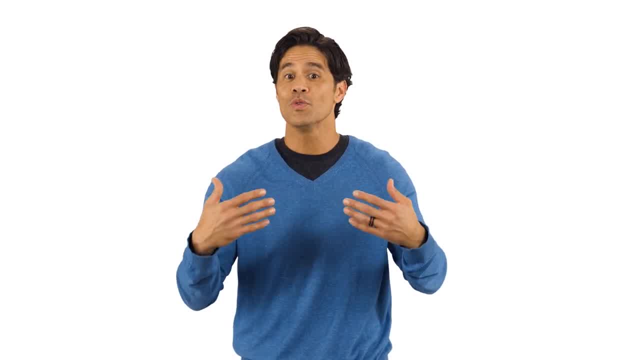 He used to lie to me about using effective negative consequences, But now that he was doing his chores and being honest about it, I wanted to reinforce his good behavior and motivate him to continue doing it. What I found is that spending time with friends is motivating to him right now. 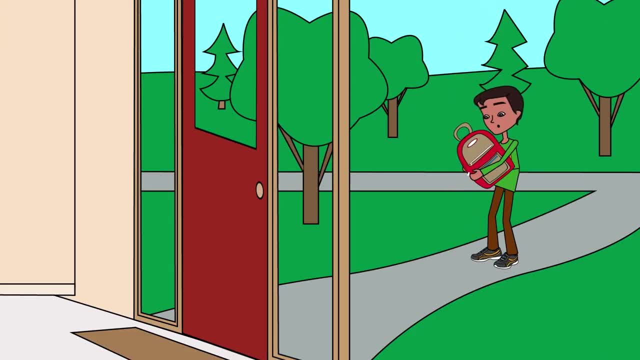 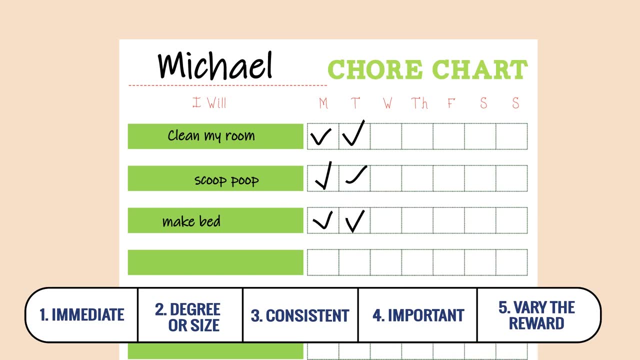 We have it set up for Michael to do chores as soon as he returns home from school, before he can do anything else. So now, as soon as Michael completes his chores, he has earned 15 minutes to text his friends to find out what is happening. 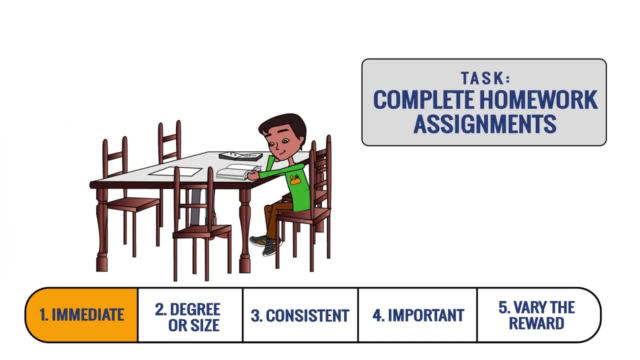 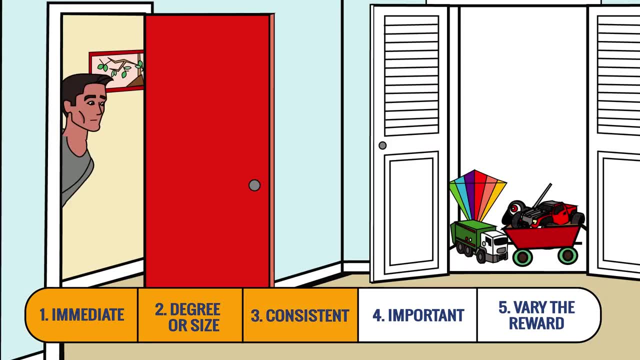 And if they want to get together later. If Michael is able to complete his homework assignments, then he is allowed two hours of time to play with friends. I was consistent by being sure he had finished his chores before allowing him to play with his friends. 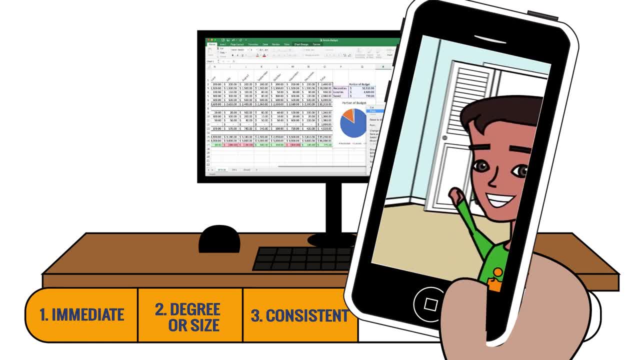 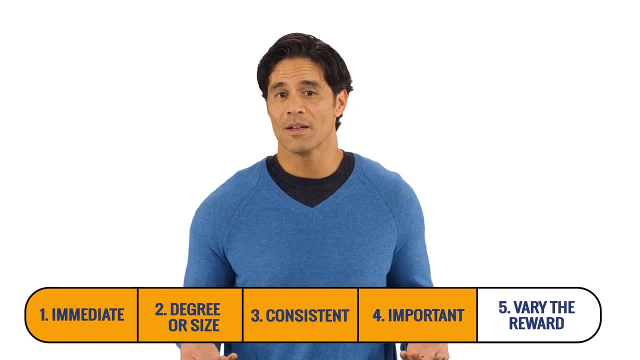 Sometimes it meant having him show me completed chores using his phone when I was at work. This reward is something that is important to him, Not only because he asks for it all the time, which he does, but because it's how he chooses to spend his free time. 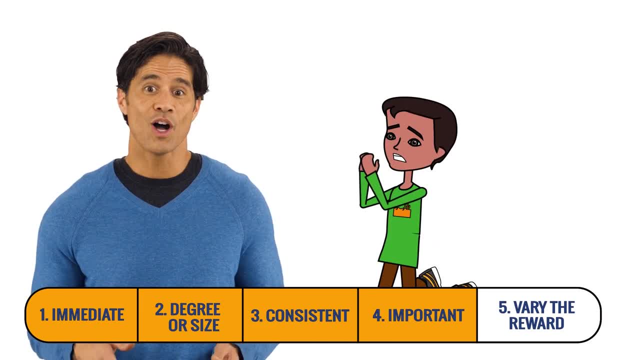 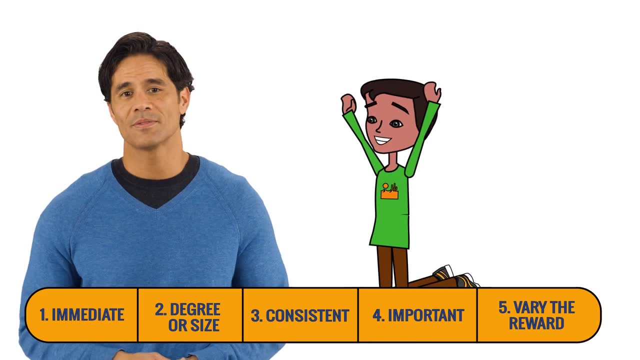 This reward works for us now, But he is already asking for more time with friends, So we will be adjusting when he can do his chores so it allows him more time with his friends. I'm willing to do this because he's getting older. 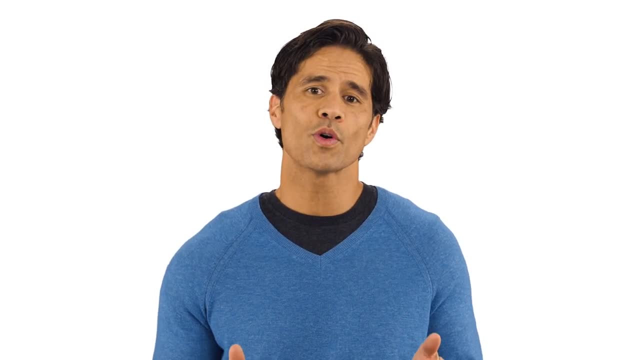 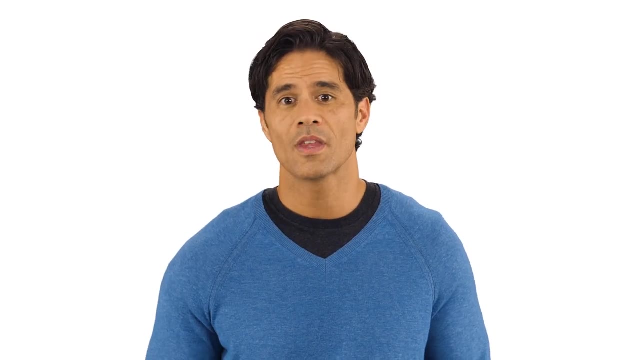 it's motivating for him and I want to reward him for positive things he's doing. If he struggles with the new arrangement, we will reassess and go back to the way it was working. I realized how important it was to use all five components with every reward. 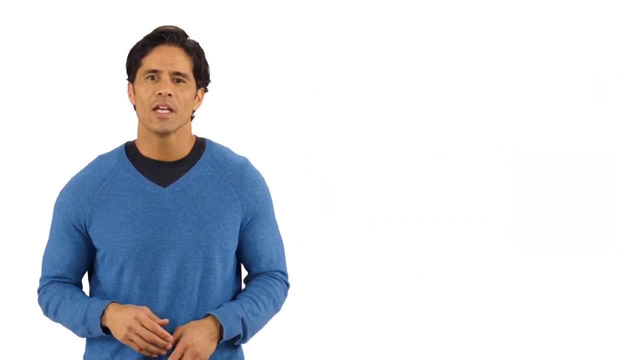 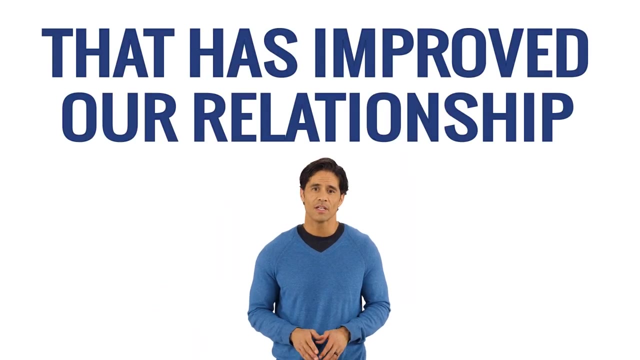 because it helped me give rewards that mean something to him. It was easier for him to keep doing something positive after being rewarded for it, And that has improved our relationship. Being a dad has its challenges. I'm not perfect, but I'm trying. 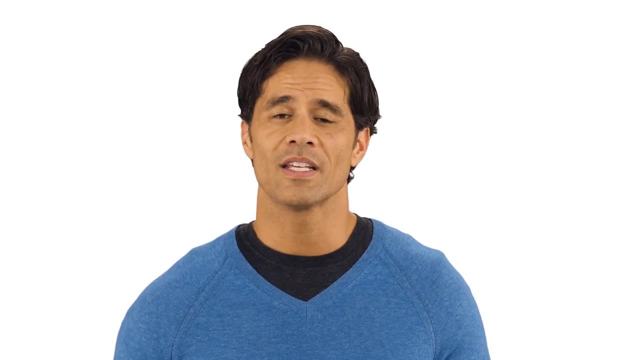 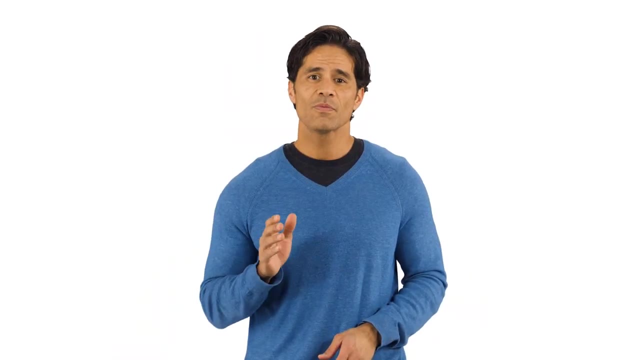 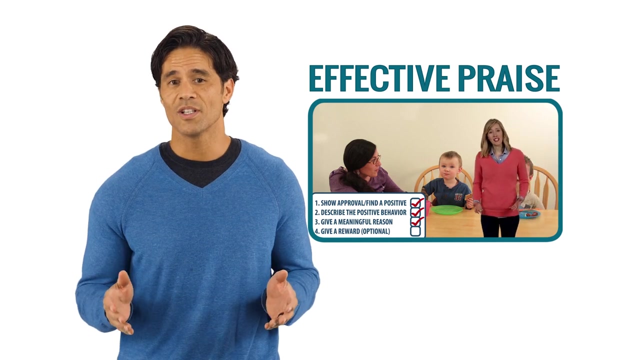 Effective positive rewards has brought me closer to my son. It has taught him the life lesson that positive behaviors can lead to positive rewards. Effective positive rewards are even more effective when combined with the skill of effective praise. You can watch this skill on the Smarter Parenting website.